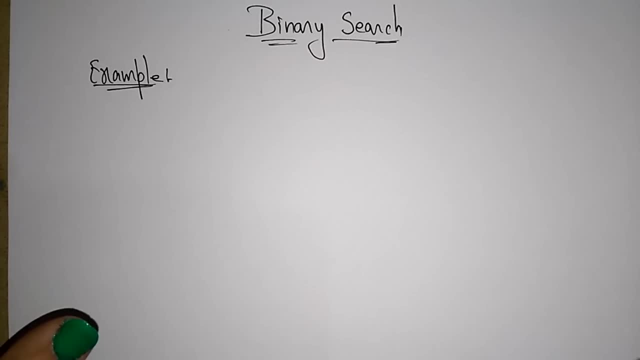 of some elements. we have to find the element. So this binary search may be successful or unsuccessful. Successful search means if the searching element is found, then you call it as a successful search. If the searching element is not found, then you call it as an unsuccessful. 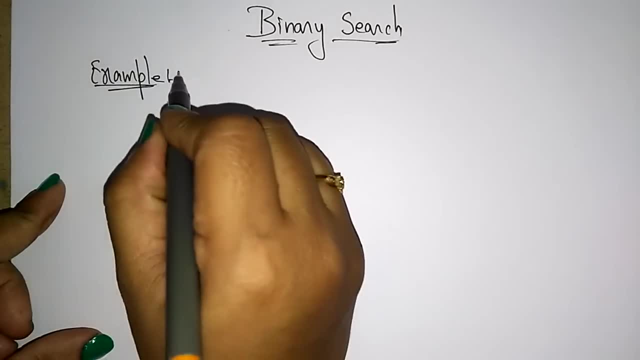 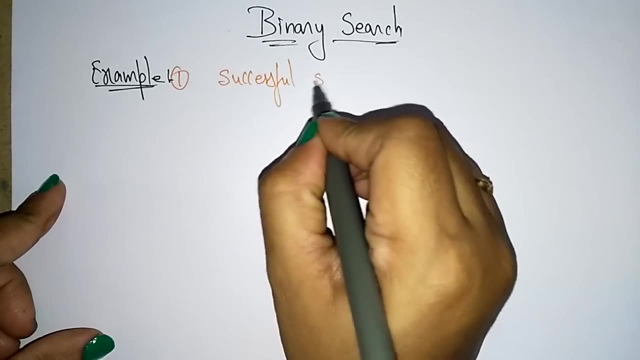 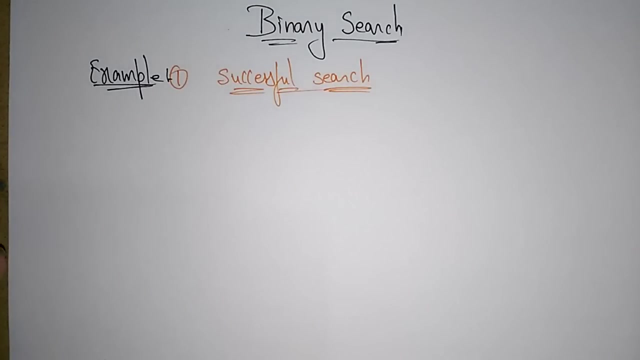 search. Now let us take two examples. So in the first example let us take the binary search of successful search Means when, whatever we are searching, so in that array we will find the search element. So in that array we will find the search element. So in that array. 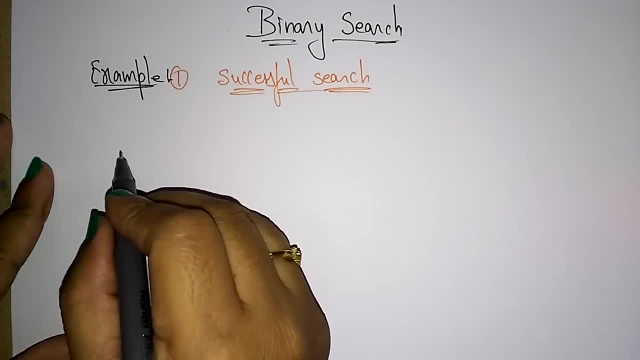 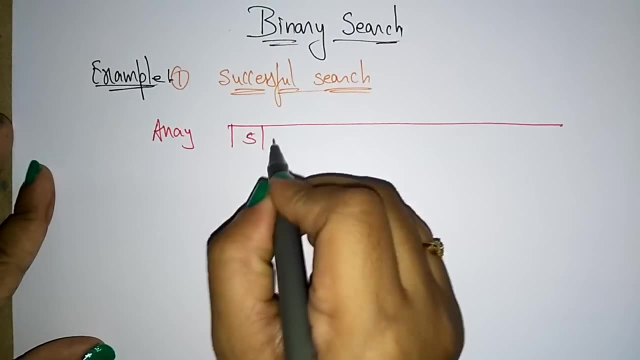 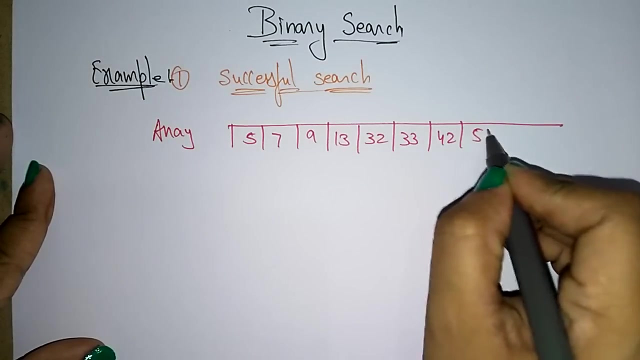 we will find an element. So let us take an array. So this is an array, Array consisting of elements 5, 7,, 9,, 13,, 32,, 33,, 42,, 54,, 56 and 88.. So one thing you have to be noted: that 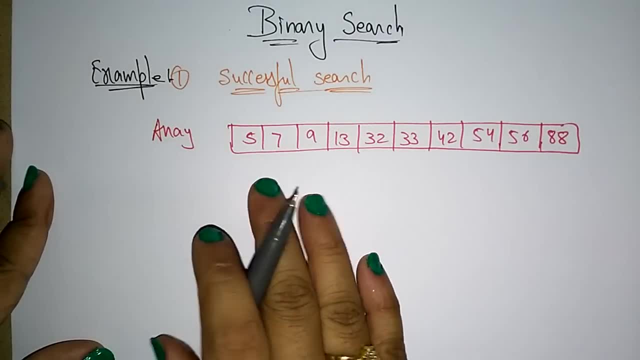 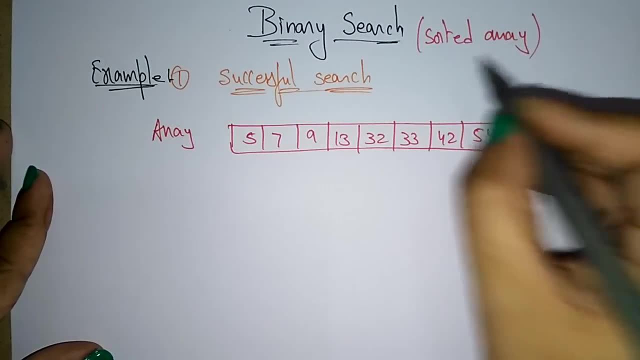 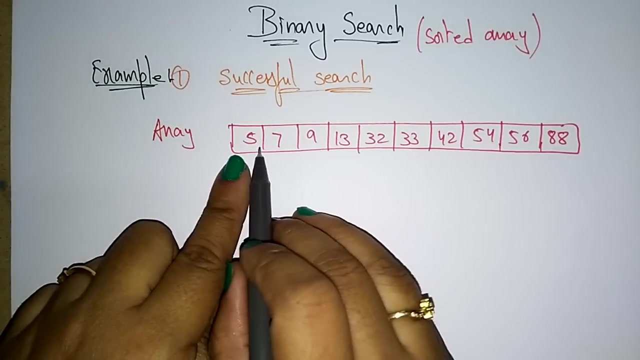 a binary search can search the element, only the sorted array. So it should be noted that a sorted array should be there. Okay, A sorted array should be there. So this is a sorted array. So all the elements are arranged in an ascending order, So 5, 7,, 9,, 13.. So, and the values? 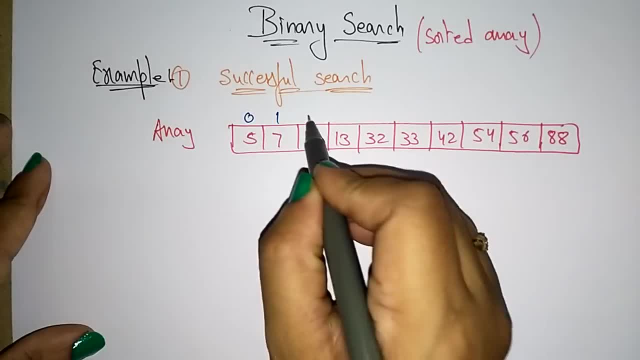 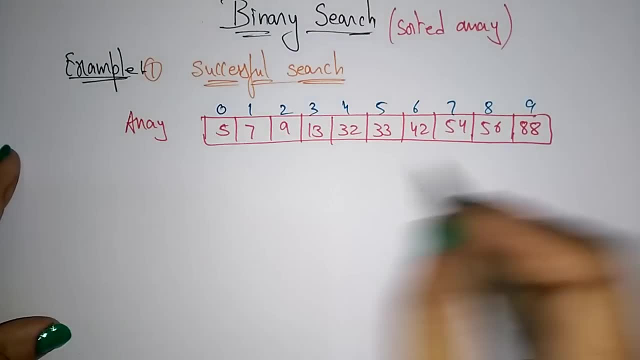 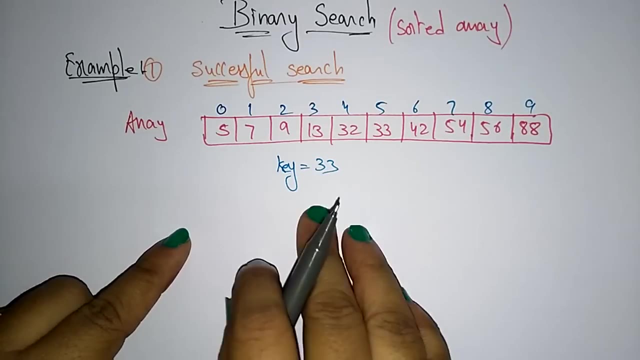 here 0,, 1,, 2,, 3,, 4,, 5,, 6,, 7,, 8, 9.. So the array size is the 9.. Let us take the key value. Key is 33.. I want to find the element 33 in this array, So how we will find? So first, 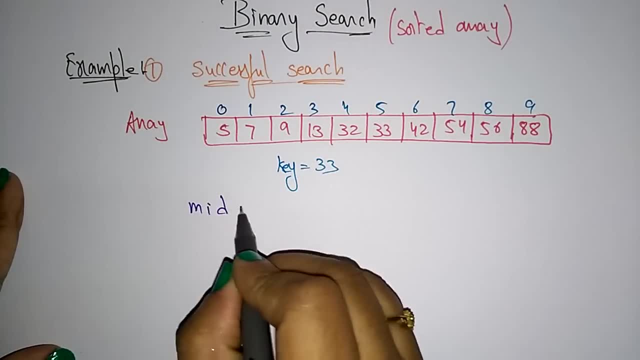 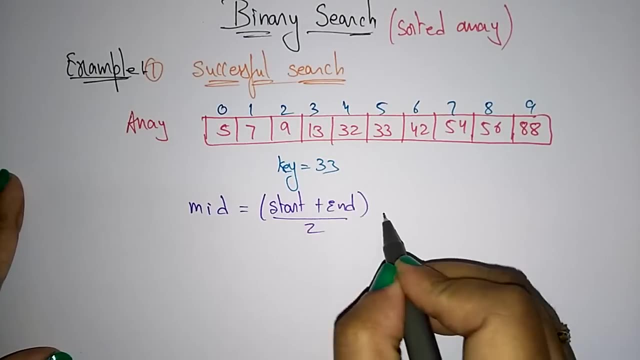 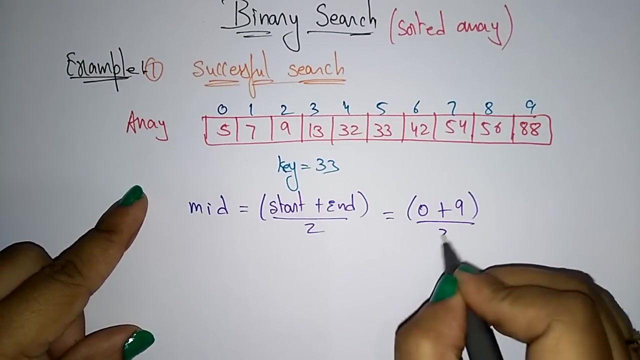 we have to divide an array That is mid is equal to start plus end by 2.. So what is the start value? Start is array 0 plus end is 9. 0 plus 9 by 2. That is 8.. So what is? 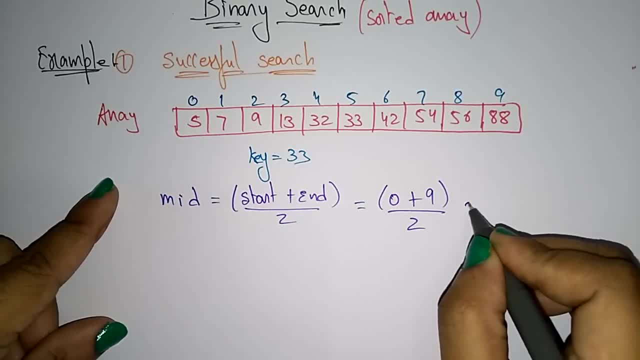 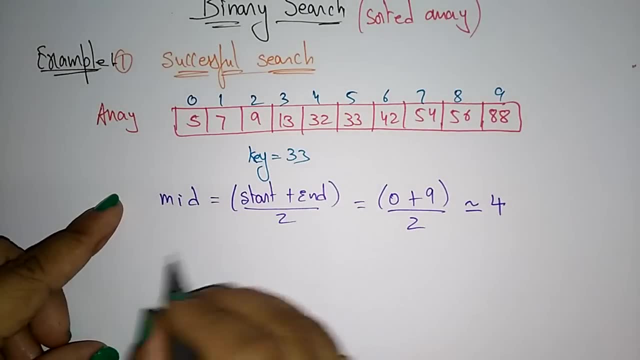 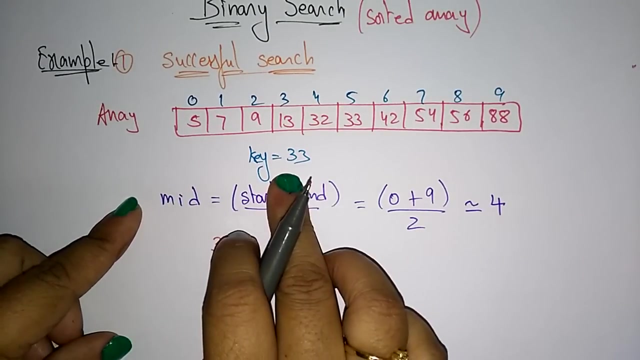 8? Means 9 by 2. That is approximately the value is 4.. So 4.. So this is here. you have to check that 33, whatever the divided value, the 33, the search key value here is greater. 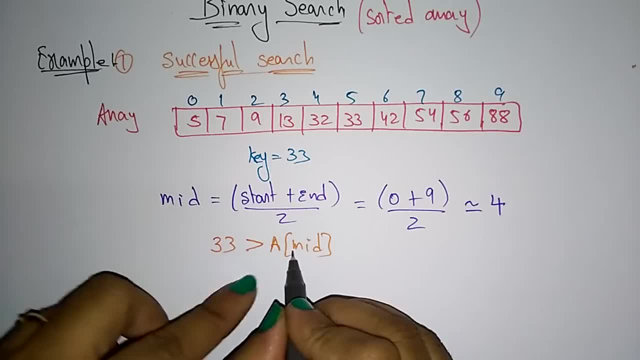 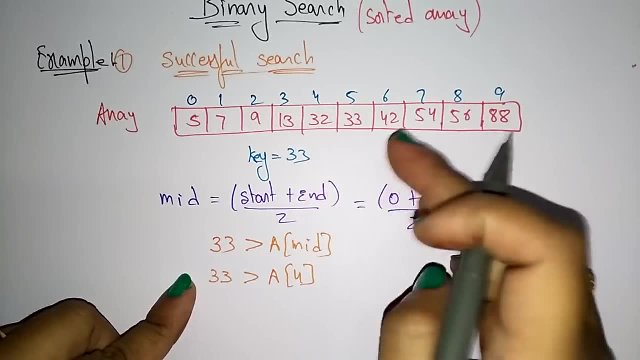 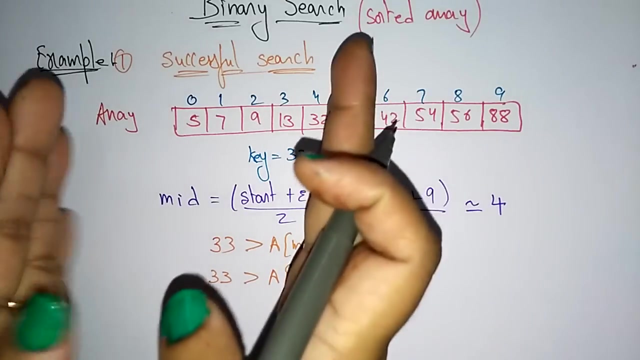 than a of mid, So mid is 4.. 33 is greater than a of 4.. So mid is 4.. So mid is 4.. So a of 4 is 32.. Okay, But the search value we want is 33.. So we have to skip this thing. 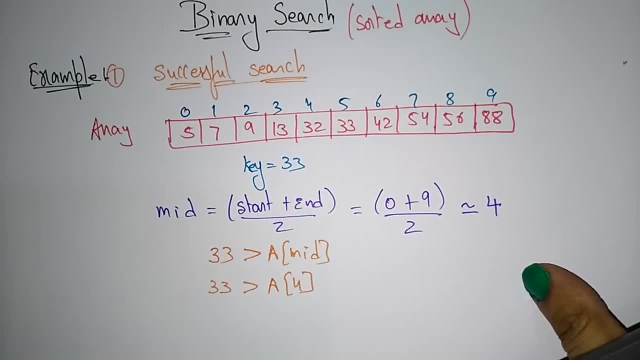 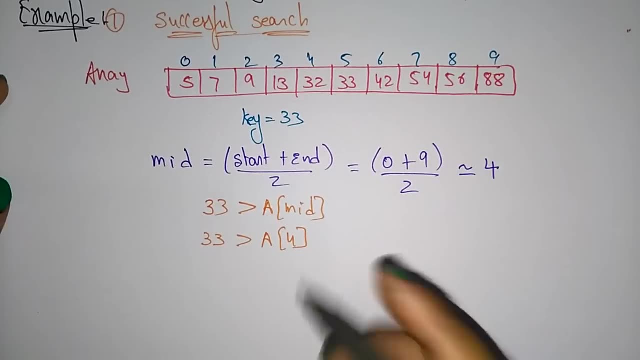 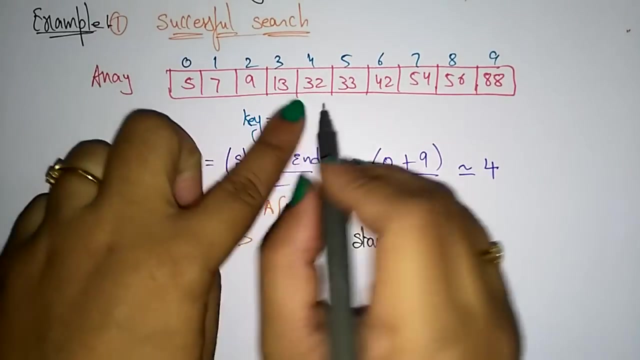 because this is greater than 33, is greater than a of 4.. Then you have to skip the left side. That means you have to take that Start is equal to mid plus 1.. That means now the start will come here. This is a start. 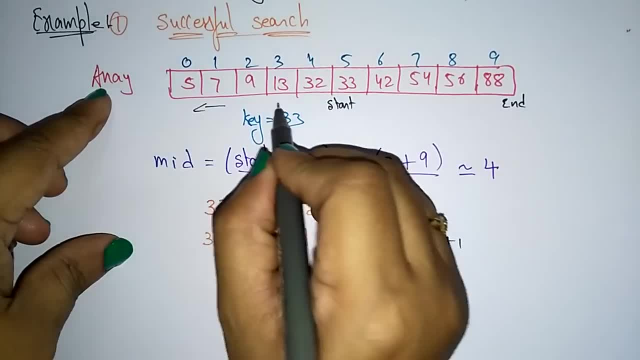 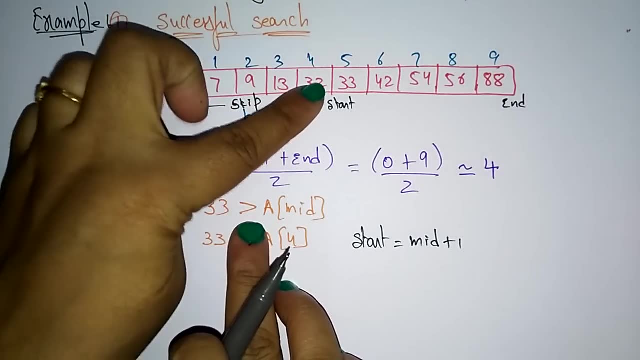 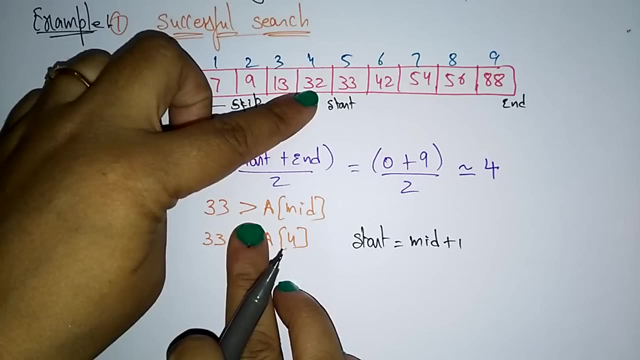 And this is the end. So we skip this. Why we are skipping this? Because the mid, the search value that is greater than a of mid. So a of mid is the 32. I got Okay, That is a 4.. The 4, a of 4 is 32.. So 33 is greater than 32.. So just skip this. Now the start. 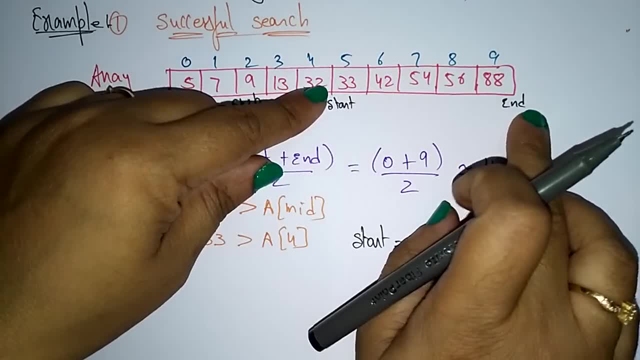 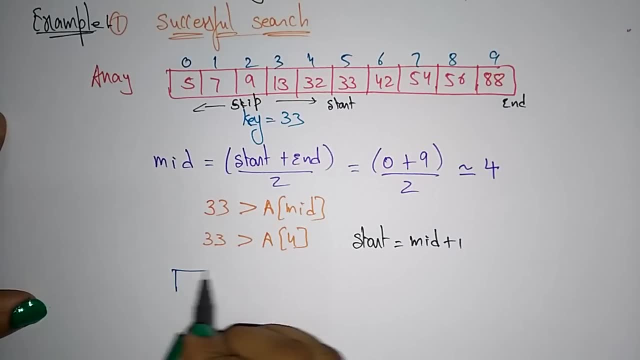 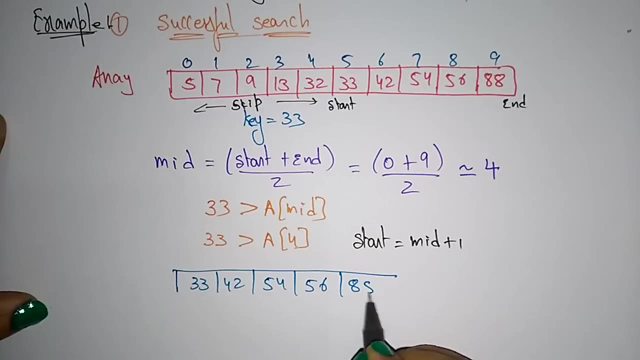 becomes this: 5 and end is 9.. Now again check. So what is the array now? So here the array is 33,, 42,, 54,, 56 and 88.. Okay, So 5,, 6,, 7,, 8,, 9.. Now again check. 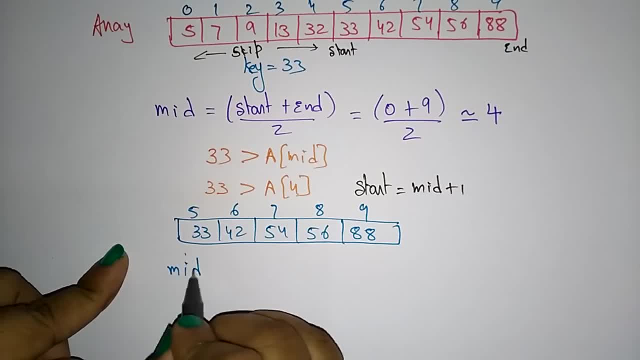 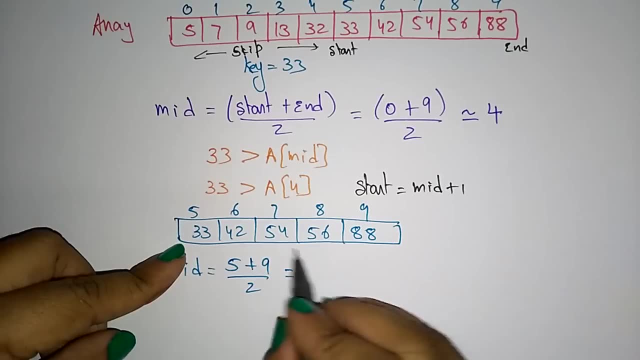 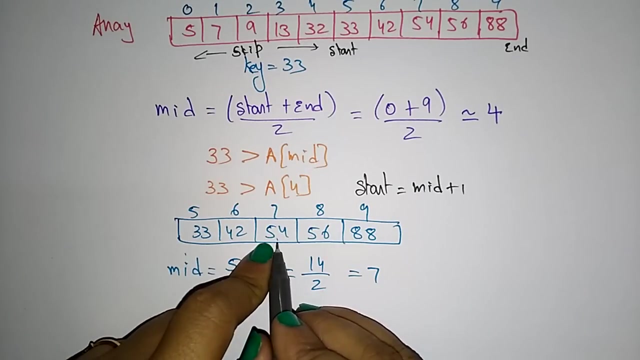 Divide the array into half. Mid is equal to start plus end. Start is 5, end is 9 by 2.. So that is 7.. So now the mid becomes 7.. So a of 7 is greater than or less than the key value. 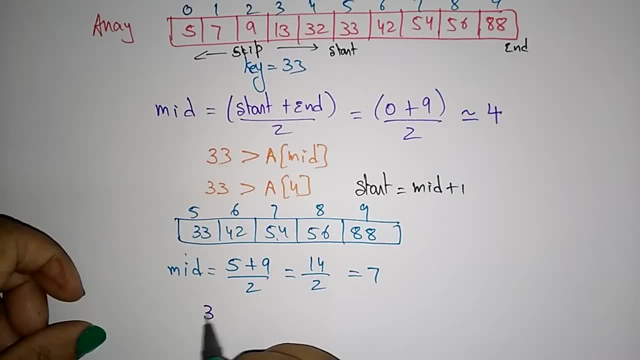 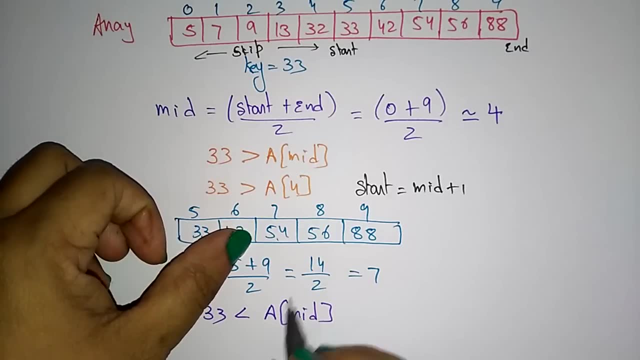 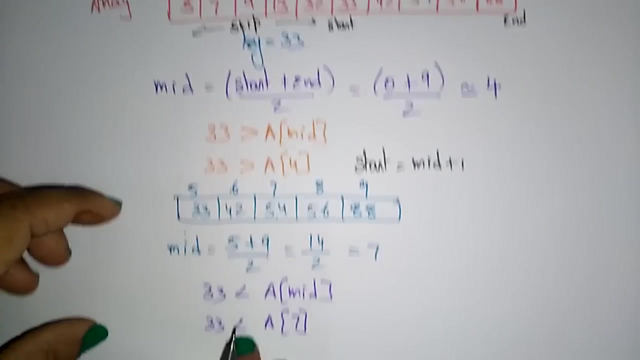 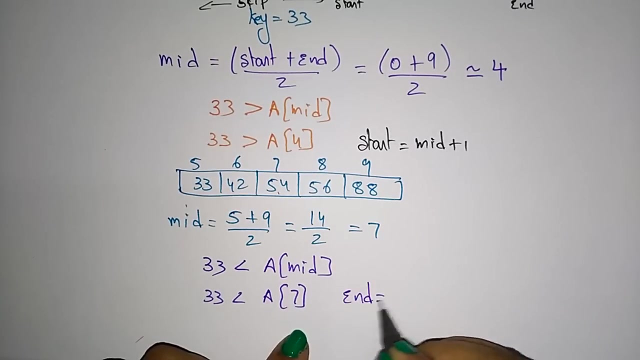 Here, 33 is less than a of mid. A of mid means a of 7.. 33 is less than a of 7.. So a of 7 is 54. So 33 is less than 54.. Okay, So now the end is mid minus 1.. Why I am taking the end as mid minus 1? Because 33 is less than a of 7.. 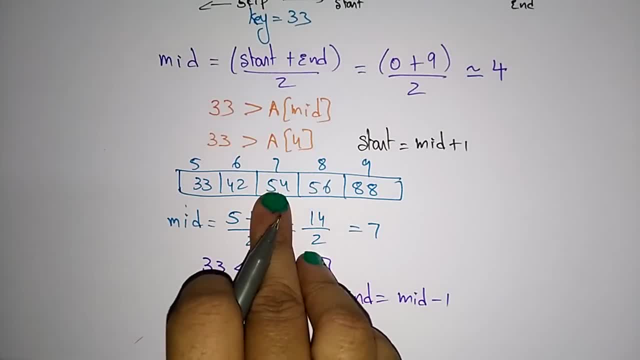 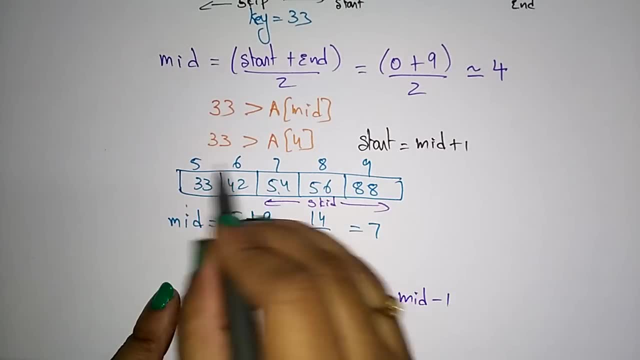 Less than a of 7 means that is, 54 is greater than, 33 is less than So you have to skip this. You have to skip this and we have to search in this left hand side. So now, here the end is. 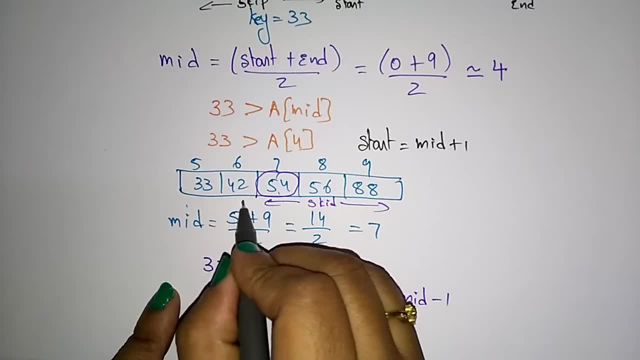 mid minus 1.. It is a middle, So let us take the end as mid minus 1.. It is a middle, So let us value so mid minus 1 and we have to search from start to mid minus 1. so that's why and is equal. 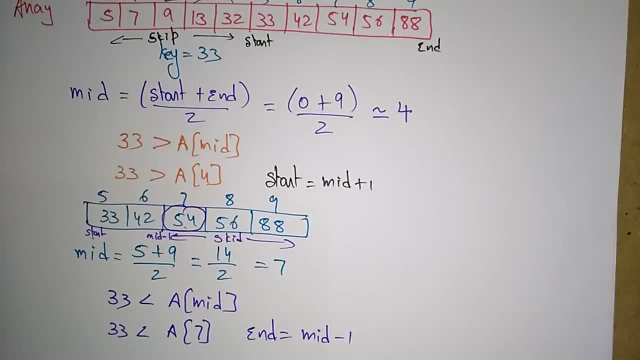 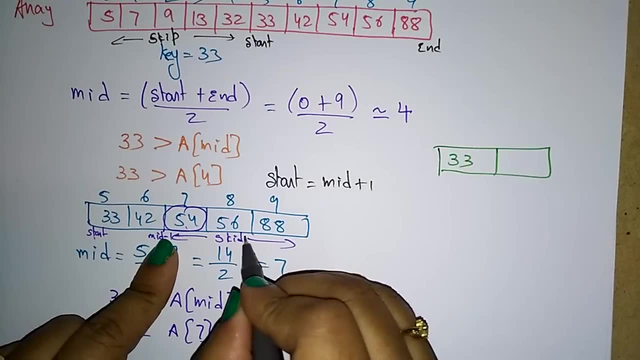 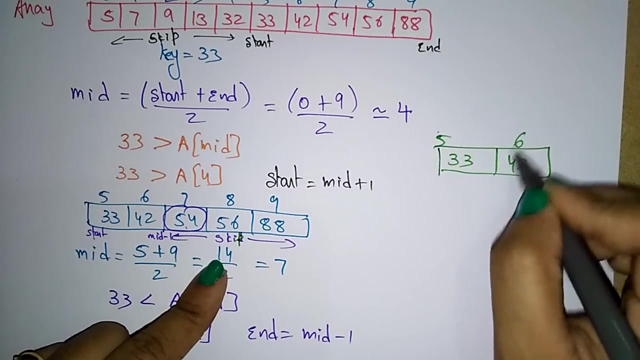 to mid minus 1. so now again the search element, these two, the array consisting of two elements now 33- just you are skipping this- 33 and 42. so 33 is 5, 42 is 6, now mid is equal to 5 plus 6 by 2. 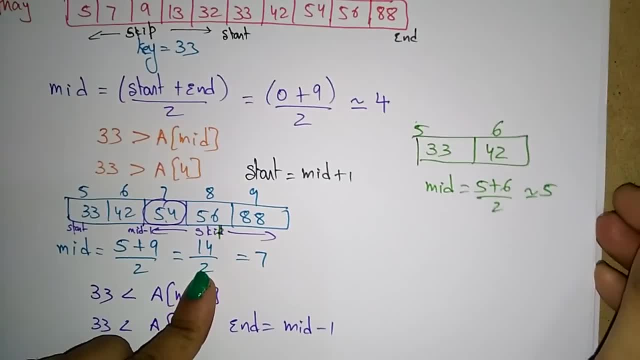 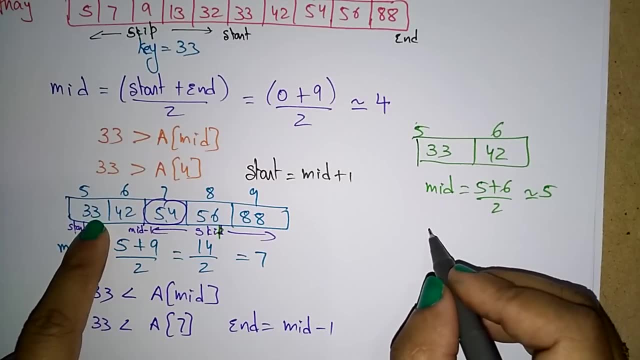 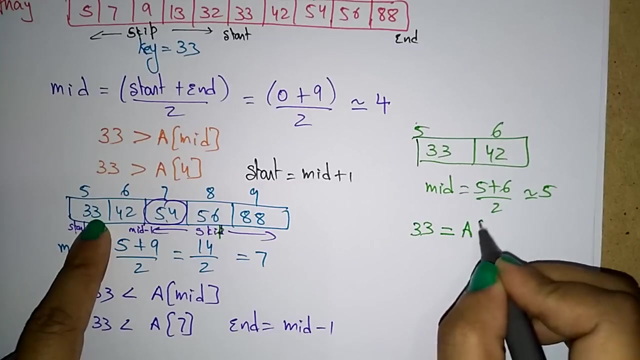 so this is approximately 5, means 11 by 2, that is approximately 5. so now the mid is 5 is a mid is equal to key value. yes, 33 is equal to a of mid. that is 33 is equal to a of 5. a of 5 value is 33. 33 is equal to 33, so 33 is. 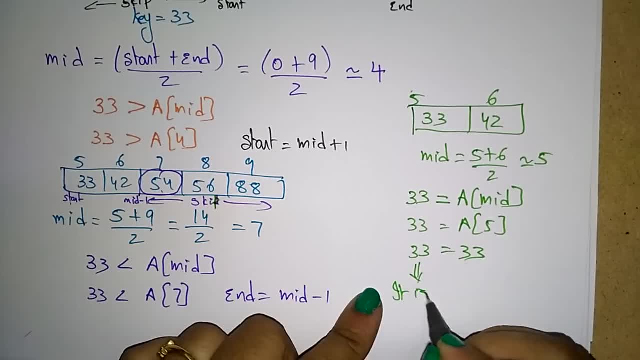 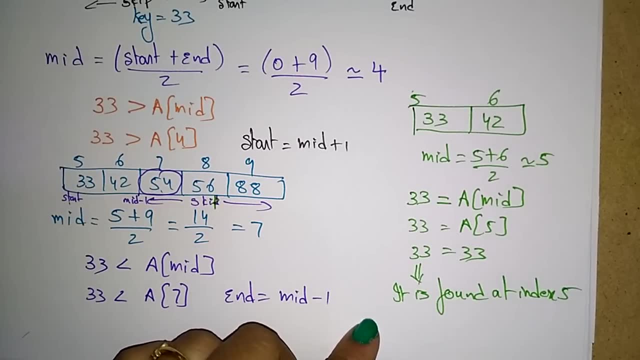 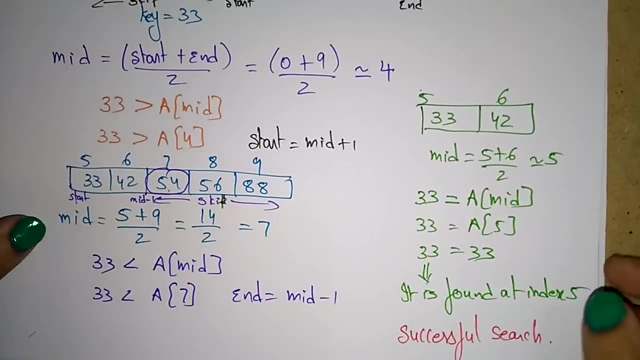 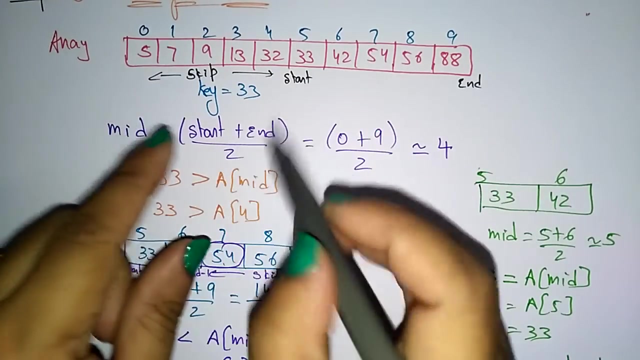 found at. it is found at index 5, then you can say it is a successful search. so this is how you have to search for element. so here the simple concept is: just take an array, so that array you have to just take the start element and the end element of an array, so 0. 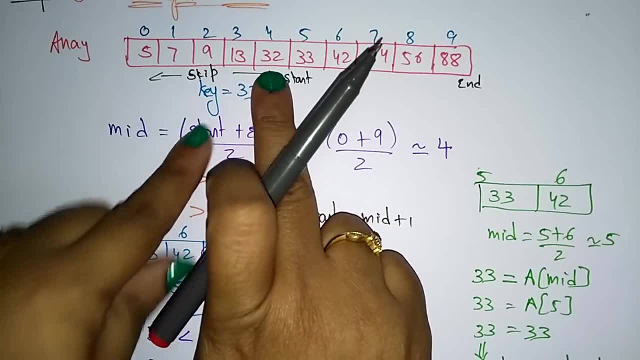 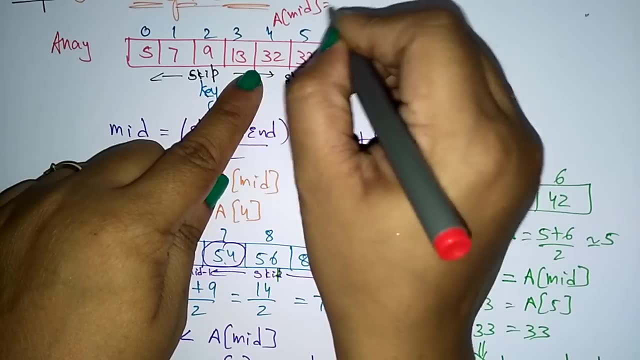 plus 9, so it is 4. so that is you get the mid element. mid element is 4. so what is a of mid, a of mid? a of mid is nothing but 32, so is 33 is greater than or equal to 32, greater than or less?